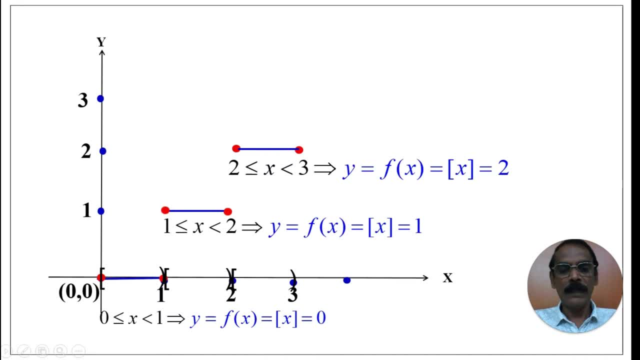 than or equals to 2, but less than 3. therefore, we are keeping closed interval here, open interval here. in this interval from 2 to 3, where 3 is excluded, The step function takes the value only 2. see, this is the value of y. this is the value of y, whose value is 2 from here to here. in this interval, from here to here, the y value is nothing but 2 only. Thus we define the step function as the value of the step function is 0 if x is greater than or equal to 0 and less than 1.. Similarly, whose value is 1 if x is greater than or equal to 1.. 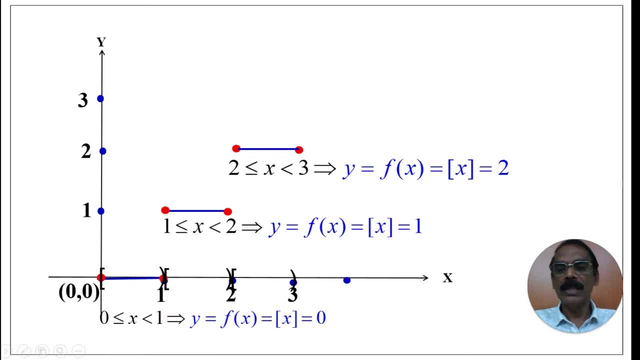 interval from here to here, the y value is nothing but 2 only. thus we define the step function as the value of the step function is 0 if x is greater than or equal to 0 and less than 1, similarly, whose value is 1 if x is greater than or equal to 1 but less than 2, and the step function 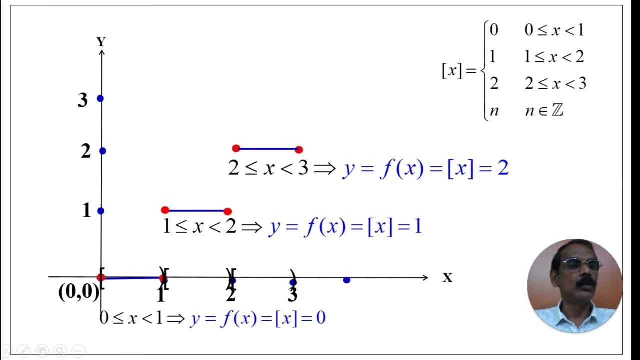 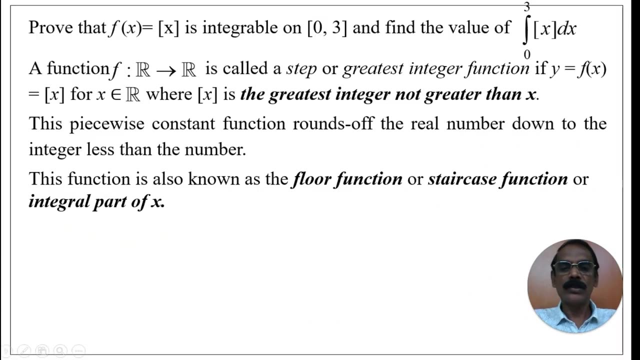 value is 2 if x is greater than or equal to 2 but less than 3 and, in general, if x is an integer, whether it is a positive integer or negative integer, or 0, the value is n only. this function is also known as floor function, or staircase function, or integral part of x, the step function. 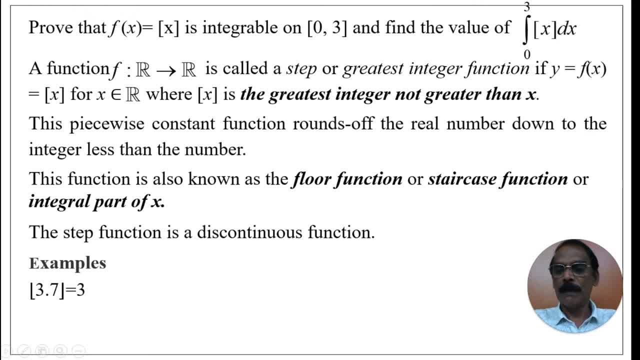 is a discontinuous function. example: what is the value of the step function if x is greater than or equal to 2 but less than 3? and, in general, of the step function 3.7, whose value is 3 because, by definition, the step function is the greatest? 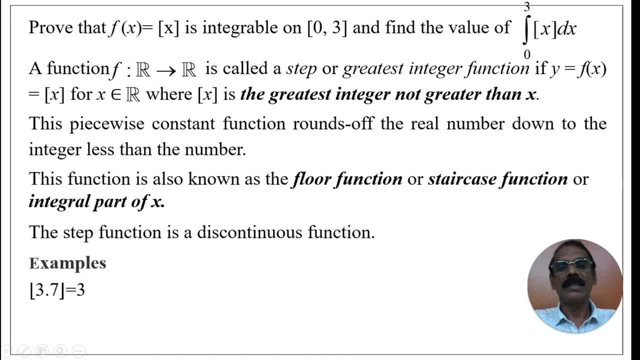 integer, but not greater than x. now, 3.7 is the value of x. now, what are the integers which are less than or equals to 3.7? the values are 3,, 2,, 1, 0, minus 1,. 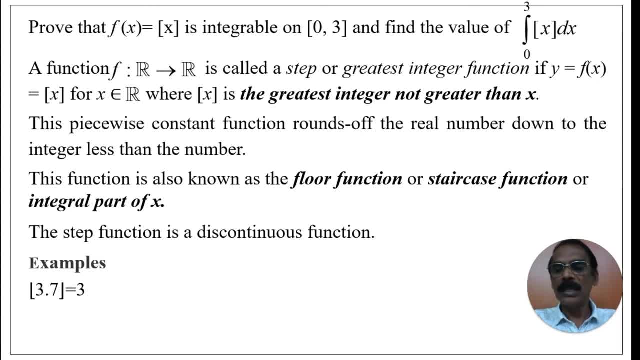 minus 2, minus 3, so on. Among these integers, which is the greatest one? 3 is the greatest one. Therefore, we have, the integral part of 3.7 is 3.. Similarly, what is the value of the step function? 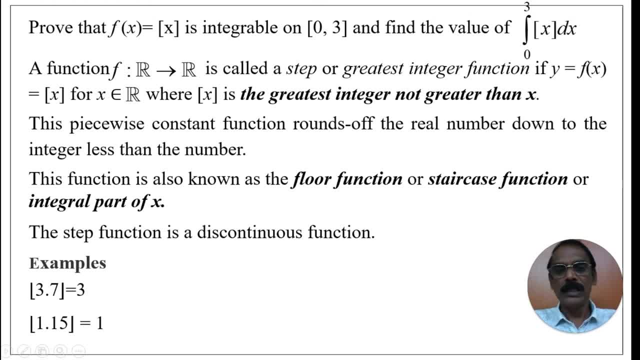 1.15?. Whose value is 1?? The reason is: x value is 1.15.. And what are the integers which are less than 1.15?? The values are 1,, 0, minus 1,, minus 2, minus 3, so on. Among these integers, which is? 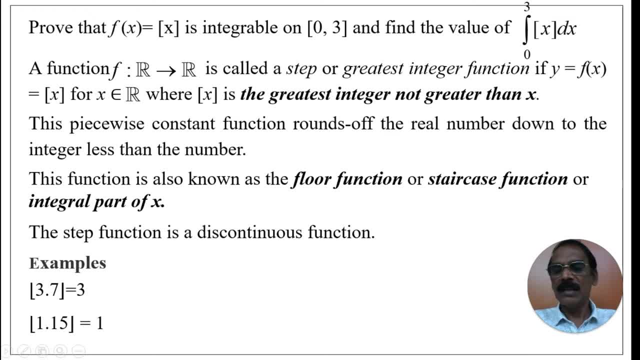 the greatest. 1 is the greatest, And hence whose value is 1?? Similarly, 4.9999 is 4.. Just now we discussed if x is an integer, the value of the step function is itself, That is, the integral. 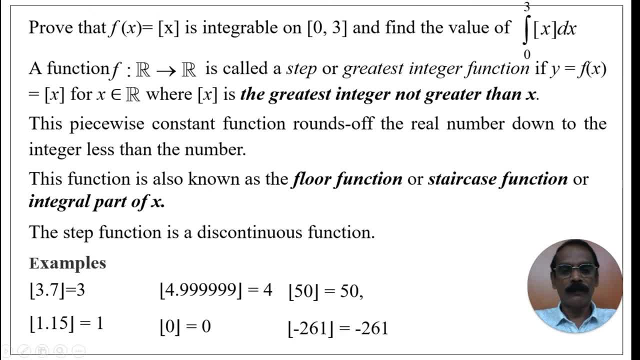 part of 0 is 0.. Similarly, integral part of 5.. 50 is 50.. Integral part of minus 2.61 is minus 2.61.. But in the case of negative value, here x takes the value minus 3.010.. What are the integers which are not greater than minus 3.014, so on. 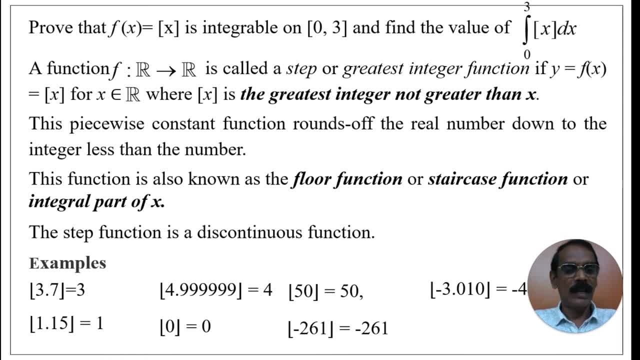 They are minus 4, minus 5, minus 6,, minus 7, minus 8.. So on, Among these, minus 4, minus 5, minus 6,, minus 7,, minus 8, so on, which is the greatest? 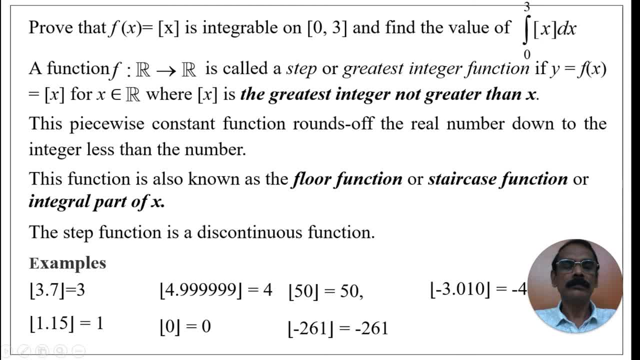 integer Minus 4.. Here, the x value is minus 3.010.. Therefore, what are the integers which are not greater than minus 3.014? They are minus 3.010.. So, what are the integers which are not greater than minus 3.014? They are. 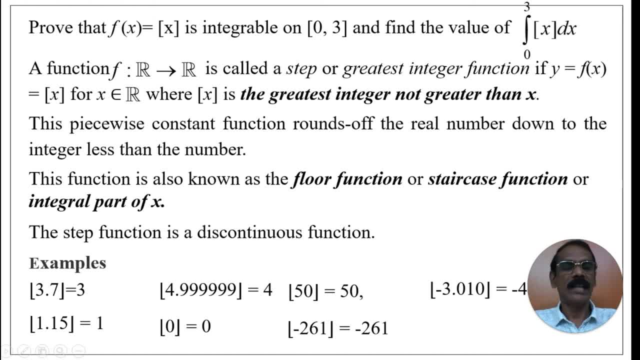 minus 4, minus 5,, minus 6,, minus 7,, minus 8, so on. Among all these integers, minus 4, minus 5,, minus 6,, minus 7,, minus 8, so on, which is the greatest one? 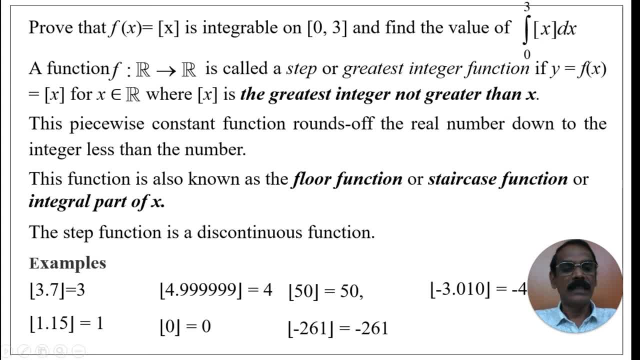 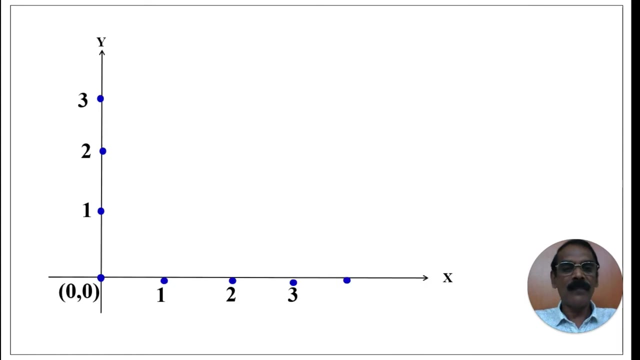 Minus 4 is the greatest one. Therefore, the integral part of minus 3.010 is minus 4.. Then, what is the value of the step function minus 1.898,, whose value is minus 2?? And this function is also called staircase function because, as in the graph- if you see the graph- 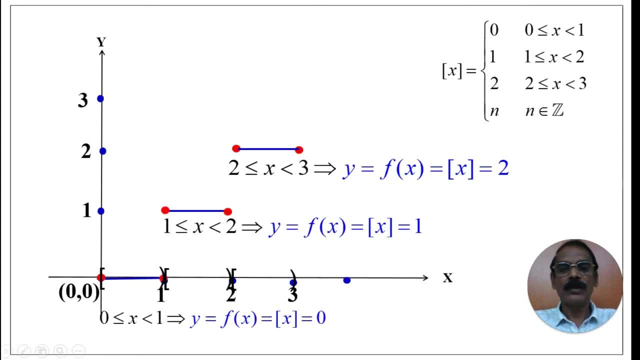 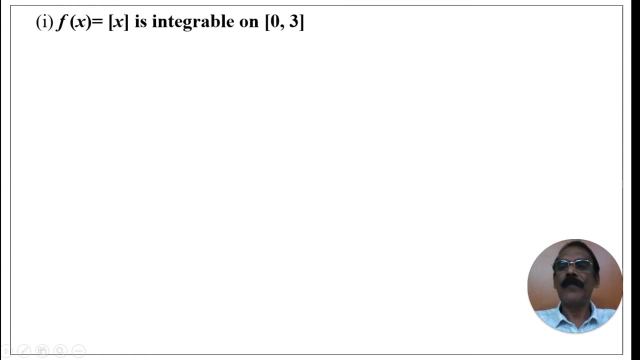 this is like a steps: 0 to 1, 1 to 2, 2 to 3 is like a step or like it's a staircase. Therefore, this function is also called step function or staircase function. We shall now show that. f of x. 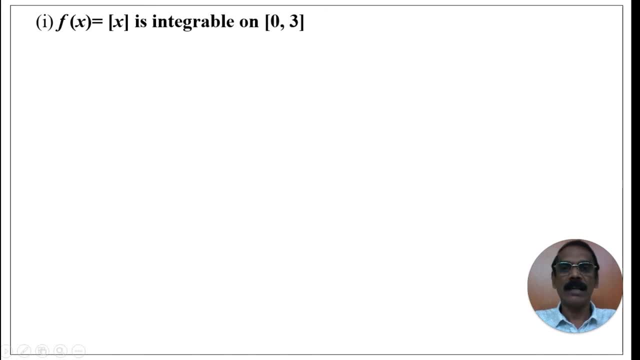 equals to the step function. x is integrable On the closed interval 0, 3.. Just now, from the graph, we come to know the value of integral part of x as 0. if x is greater than or equal to 0 and less than 1,, whose value is 1, if. 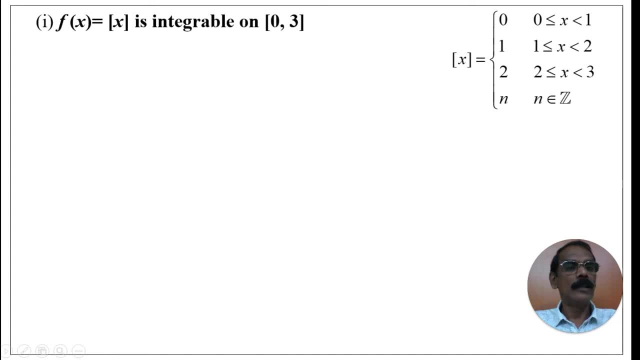 x is greater than or equal to 1 and less than 2, whose value is 2 if x value is greater than or equal to 2 and less than 3.. Therefore, clearly, 0 less than or equal to x less than. 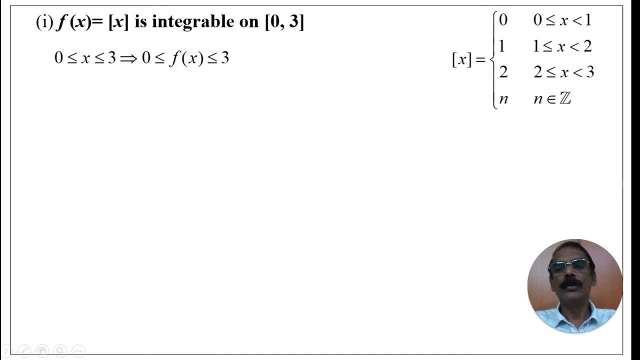 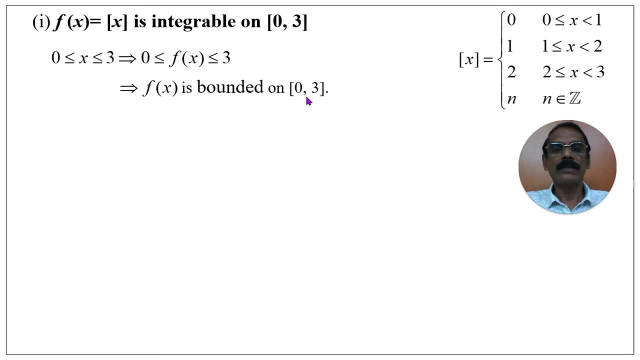 or equal to 3 implies 0 less than or equal to x. less than or equal to 3 implies f of x. value is from 0 to 3.. This implies f of x is bounded on the closed interval 0, 3.. Therefore, f has only two points of discontinuity, namely x is equals to 1 and x is equal to. 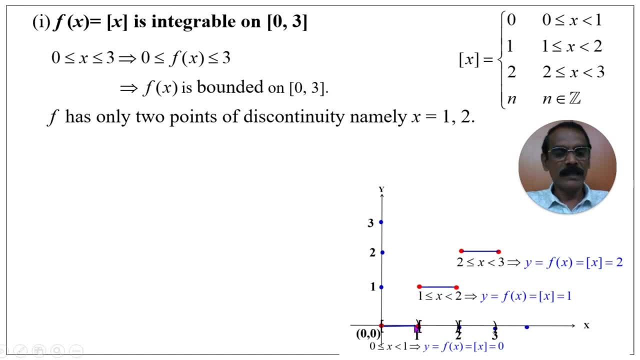 2.. This is 1.. The graph is, from here to here, discontinuous, but it has a break here, That is, it is discontinuous at 1.. From here to here, it is discontinuous. Again, there is a break. That is discontinuous. Therefore, from here to here, it is discontinuous, Therefore. 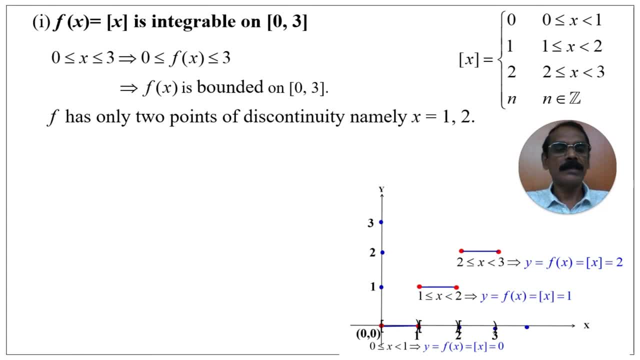 this function is discontinuous. Therefore, the step function is always discontinuous at integers And hence, and this function has two points of discontinuity, namely 1, and 2.. Therefore, by one of the classes of functions that are Riemann, integrable here. 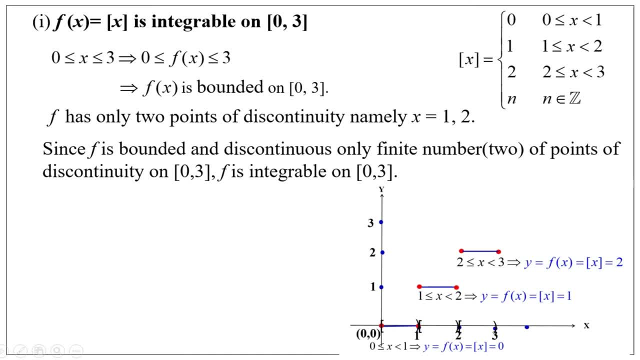 f is bounded and discontinuous Only finite number of points, that is, two points of discontinuity on the closed interval: 0, 3.. F is integrable on the closed interval: 0, 3.. Or 0 less than or equal to x less than or equal to 3 implies 0 less than or equal to 3 implies 0 less than. 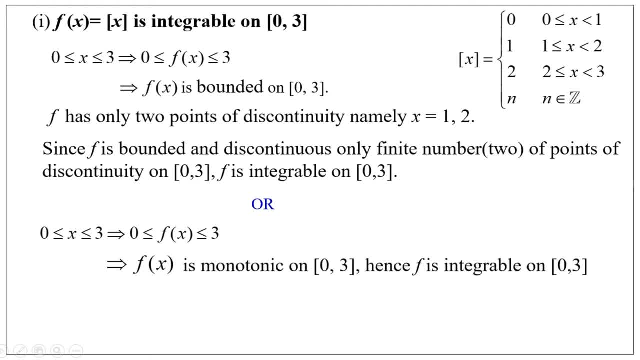 equals to f of x, lesser equal to 3.. That is, this function is monotonic on the closed interval 0 to 3, because the x value is increasing from 0 to 3.. Same way, f of x value is also increasing from 0. 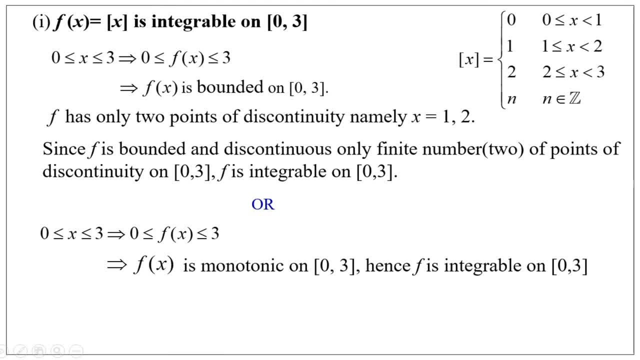 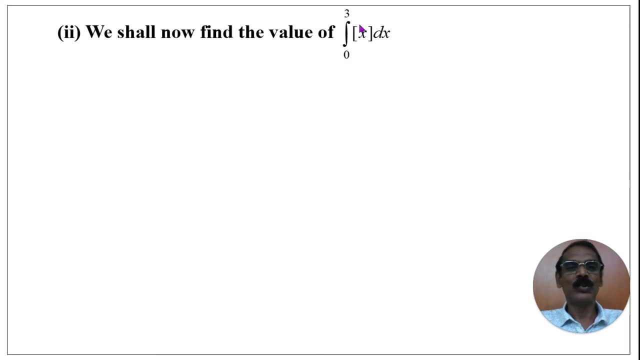 to 3.. Therefore it is a increasing function and it is a monotonic function. Hence f is remon integrable on the closed interval 0 comma 3.. We shall now find the value of integral from 0 to 3, integral part of x into dx. Integral from 0 to 3, step function x, dx can be written as integral. 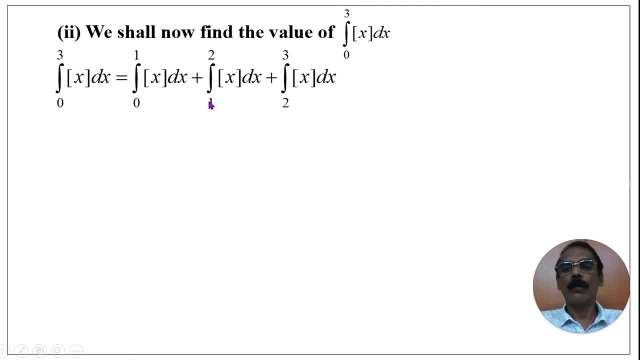 from 0 to 1, plus integral from 1 to 2, plus integral from 2 to 3.. And these are the values of the integral from 0 to 3.. So this is the integral from 0 to 3.. So this is the integral from 0 to. 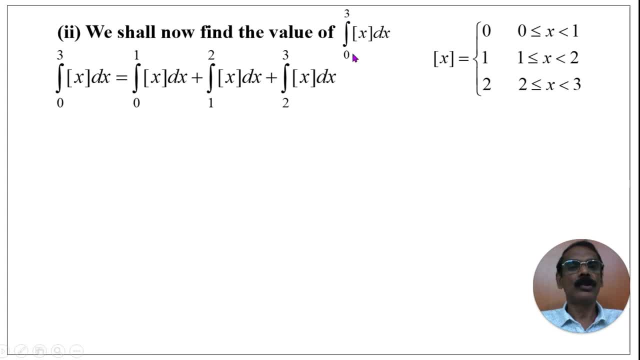 3 integral part of x in the interval 0 to 3.. Therefore, that is equals to integral. from 0 to 1 integral part of x. dx value is 0. That is when x takes value from 0 to 1, excluding 1,. 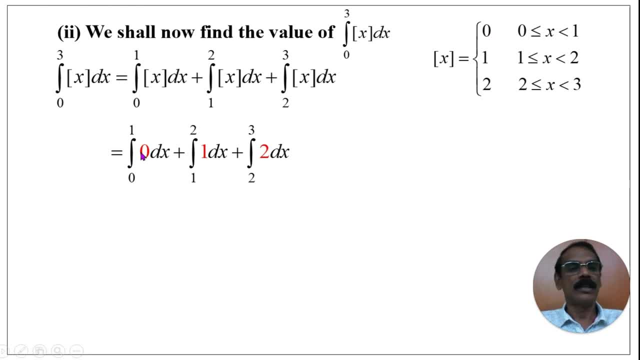 the functional value is 0.. Therefore 0.. When x is greater than or equal to 1, less than 2, this step function value is 1.. Therefore, this value is replaced by 1.. Therefore, this value is replaced by 1.. Therefore, this value is replaced by 1.. 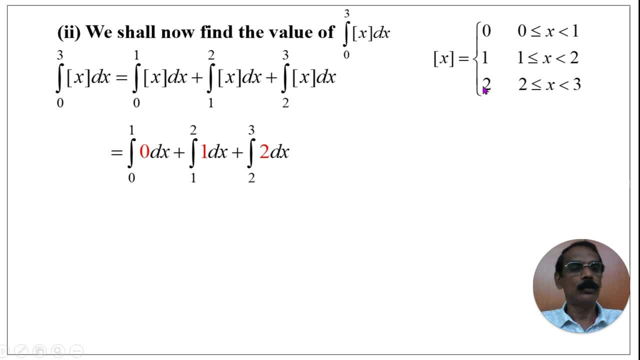 Similarly, this value is replaced by 2.. The shortcut for this is integral from a to b. integral part of x. dx is equals to integral from a to b. a dx, That is simply write. the lower limit of the integral 0 is the lower value 0, 1, 1, 2, 2.. That is equals to this value, 0 plus integrate dx. 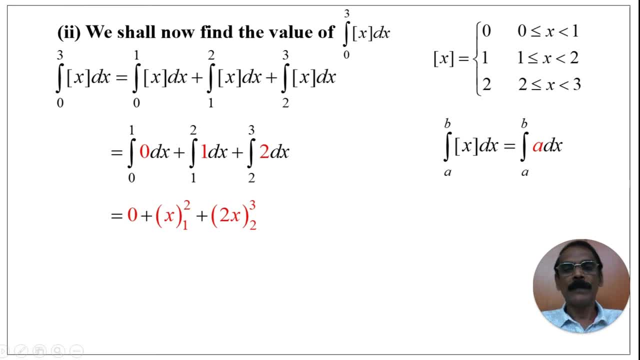 we get x. Apply the limit from 1 to 2.. If we integrate dx, we get 2.. Therefore, 2x. apply the limit from 2 to 3.. That is equal to 2 minus 1 plus 2 into 3 minus 2.. This is equals to 1 plus. 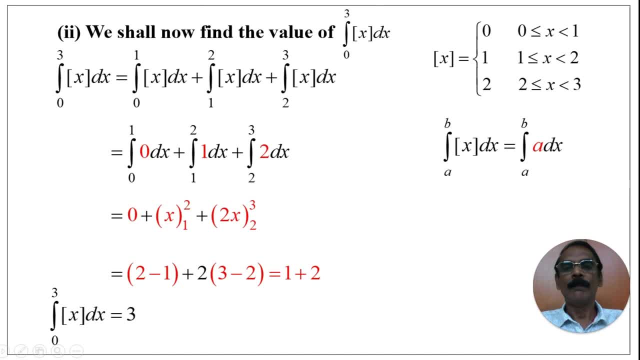 2 into 1, 2. That is equals to 3.. Therefore, the value of this integral 0 to 3 step function x, dx is equals to 3.. The shortcut for this type of problem is integral from 0 to 3. That is equal to 2.. Therefore, the value of this integral 0 to 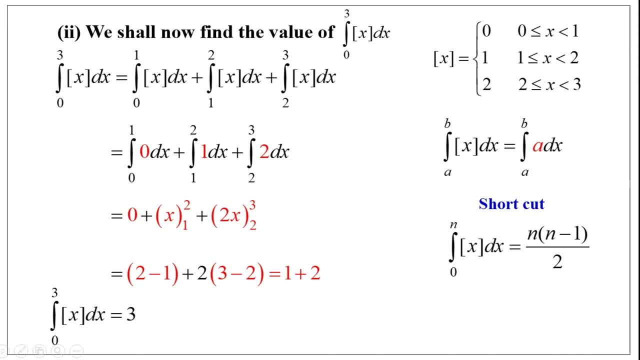 n step function. x dx is equals to n into n minus 1 by 2.. Therefore, integral from 0 to 3, integral part of x dx, is equals to n is 3.. That is equals to 3 into 3 minus 1 by 2. That is 3 into 2 by 2.. 2 will get cancelled, whose value is? 3.. 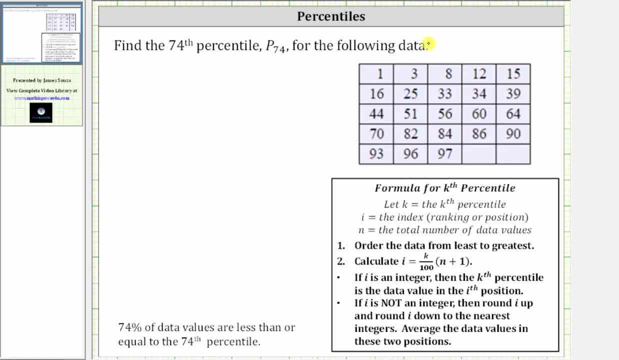 We were asked to find the 74th percentile for the following data: There is more than one method for determining a percentile. In our class, we'll use the method outlined below, where we let k equal the kth percentile, which, in our case, because we are looking, 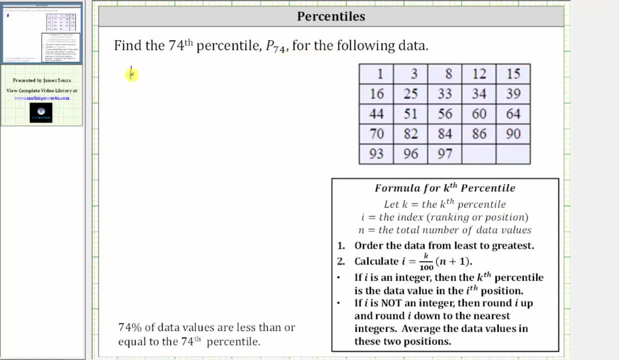 for the 74th percentile: k equals 74,. i equals the index, which is also referred to as the ranking or position of a given data value, and n is equal to the total number of data values. because we have 23 data values, n equals 23.. 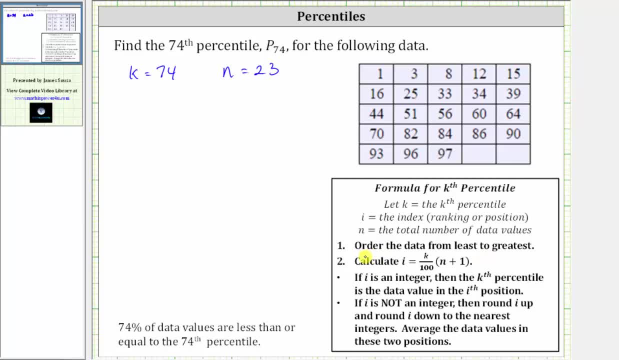 And now to find the 74th percentile. the first step is to order the data from least to greatest. In our case, though, looking at the table, the data values are already in order from least to greatest in rows. Step two: we calculate i, which is equal to k divided by 100. 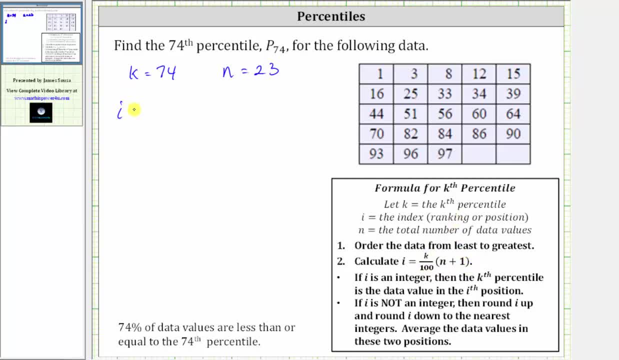 times the quantity n plus one. So i is equal to k divided by 100, is 74 divided by 100,. and then times the quantity n plus one, which in our case gives us the quantity 23 plus one. Simplifying 74 divided by 100 is equal to 0.74,.